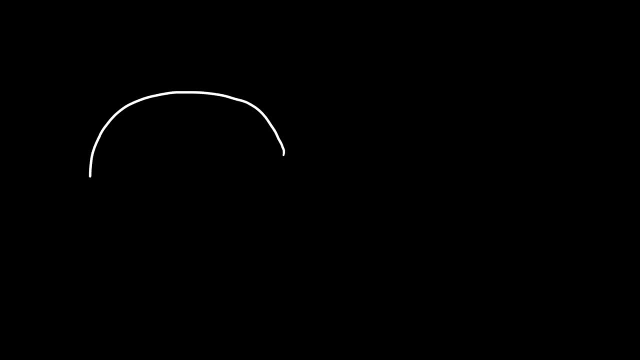 Let's begin our discussion with a circle. So let's say: this is the center of the circle and let's put some points to it. Let's call this point A. This is going to be B, D, E. Let's call this X and point C. 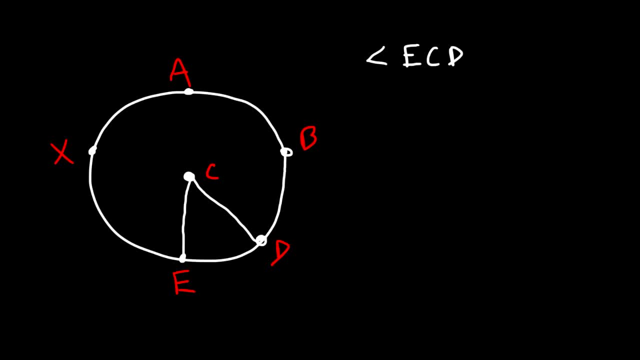 Angle E C D is known as the center of the circle. Angle E C D is known as a central angle. A central angle is an angle where the vertex of the angle is the center of the circle. So E C D is a central angle. Now let's say, if this angle is 40 degrees, 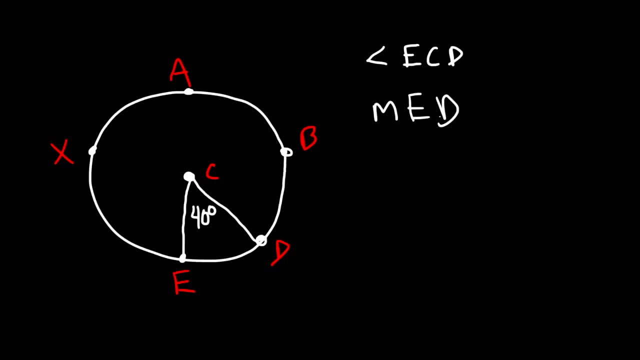 What is the measure of arc E D? So what's the angle measure of this arc? The angle measure of the intersection, The angle measure of the intercepted arc, is equal to the central angle. So that's going to be- Actually, let me redraw that- That's going to be 40 degrees. 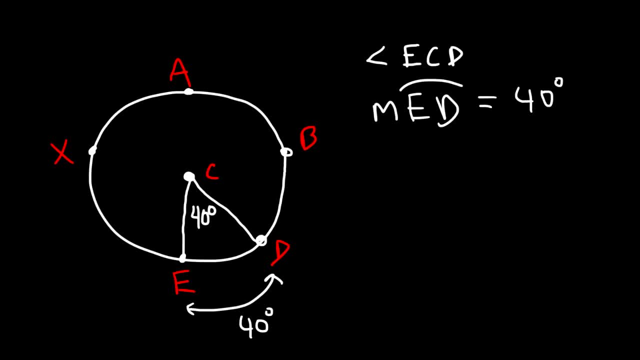 So the measure of arc E D is 40. And if we draw a segment between E D that's a chord. So make sure you know the difference between a segment and the measure of an arc. Now, arc E D: is it a minor arc or a major arc? 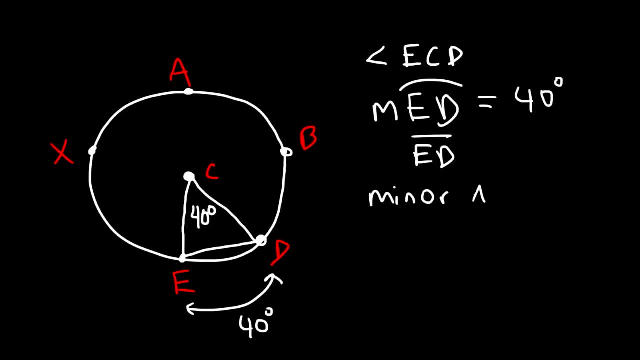 A minor arc has an angle that's less than 180.. A major arc has an angle that's greater than 180.. So because arc E D is part of the central angle and it's less than 180, that arc is a minor arc. 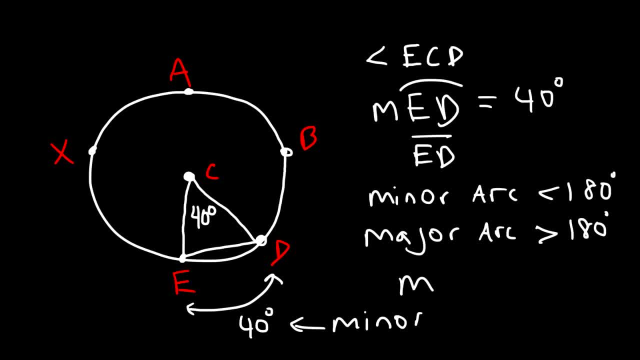 Now what about, let's say, the measure of arc E X D? So notice that we have three points instead of two points. So arc E D is right here. It's the shortest path between E and D on the circle. 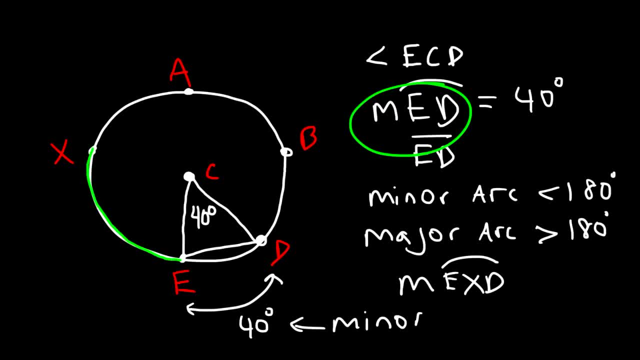 But arc E, X, D. we have to start from E, go towards X until we get back to D, Notice that it's much greater than 180.. The third point is to indicate direction. So, starting from E, we go to the second point and then towards the third point. 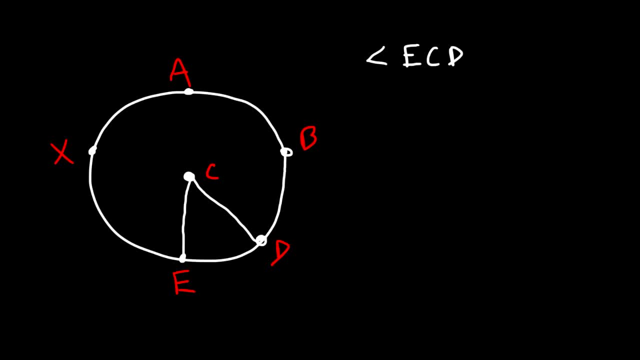 Angle E C D is known as the center of the circle. Angle E C D is known as a central angle. A central angle is an angle where the vertex of the angle is the center of the circle. So E C D is a central angle. Now let's say, if this angle is 40 degrees, 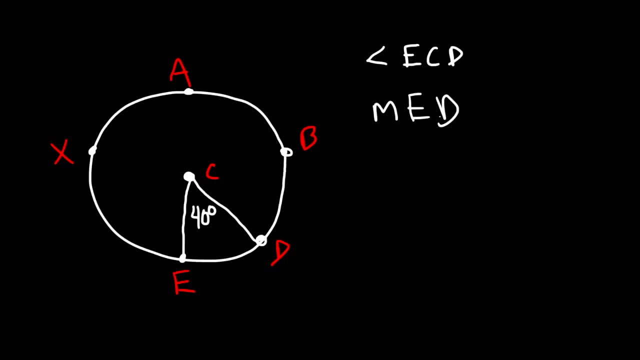 What is the measure of arc E D? So what's the angle measure of this arc? The angle measure of the intersection, The angle measure of the intercepted arc, is equal to the central angle. So that's going to be- Actually, let me redraw that- That's going to be 40 degrees. 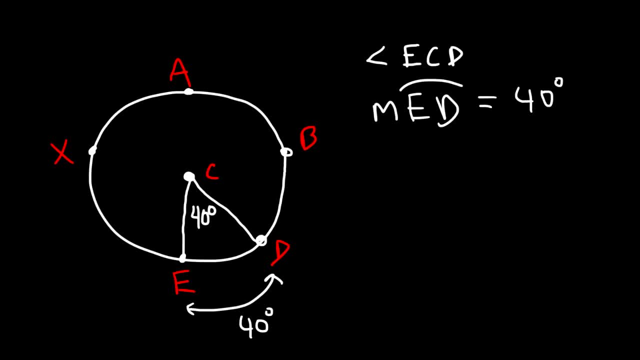 So the measure of arc E D is 40. And if we draw a segment between E D that's a chord. So make sure you know the difference between a segment and the measure of an arc. Now, arc E D: is it a minor arc or a major arc? 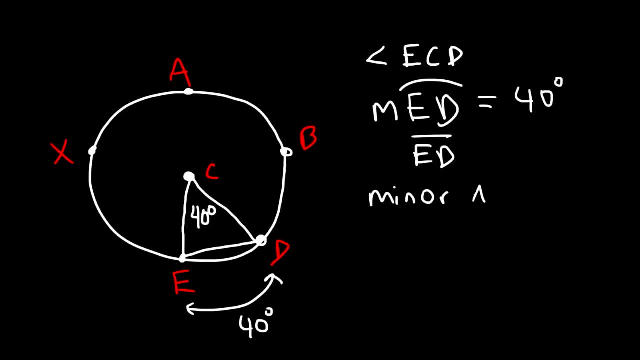 A minor arc has an angle that's less than 180.. A major arc has an angle that's greater than 180.. So because arc E D is part of the central angle and it's less than 180, that arc is a minor arc. 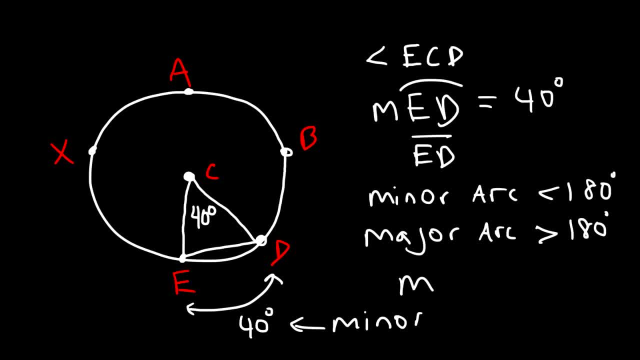 Now what about, let's say, the measure of arc E X D? So notice that we have three points instead of two points. So arc E D is right here. It's the shortest path between E and D on the circle. 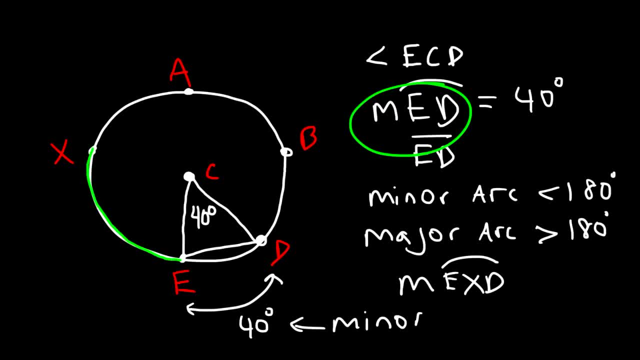 But arc E, X, D. we have to start from E, go towards X until we get back to D, Notice that it's much greater than 180.. The third point is to indicate direction. So, starting from E, we go to the second point and then towards the third point. 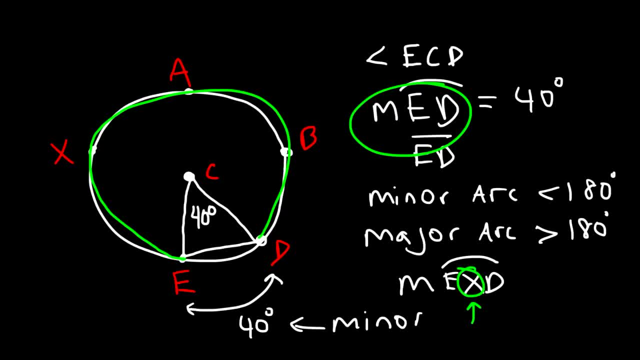 So the middle point, I mean the second point, that extra point is to help us know where we're going, And so that defines the major arc. To calculate the measure of the major arc, it's simply 360 minus the minor arc. 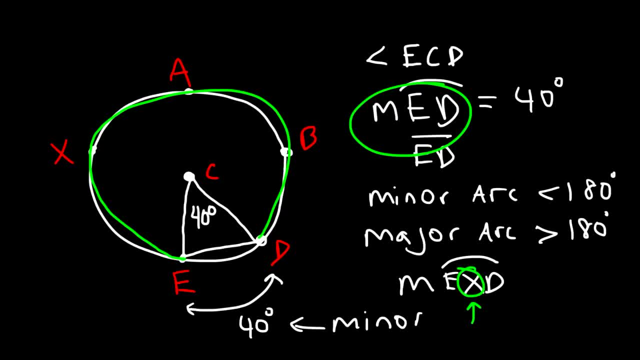 So the middle point, I mean the second point, that extra point is to help us know where we're going, And so that defines the major arc. To calculate the measure of the major arc, it's simply 360 minus the minor arc. 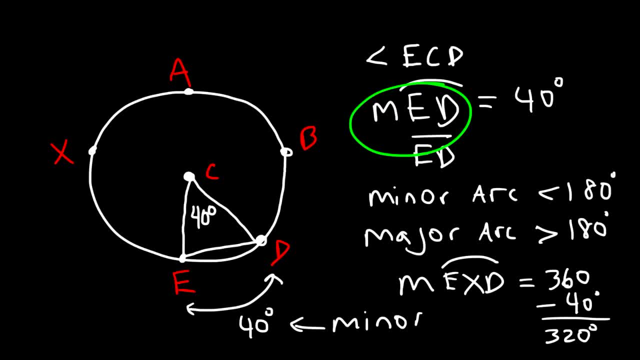 So the measure of arc E, X, D is 320 degrees. So from here all the way to the other side, that's 320 degrees. A full circle is 360.. So we've seen that a minor arc is less than 180, and a major arc is greater than 180. 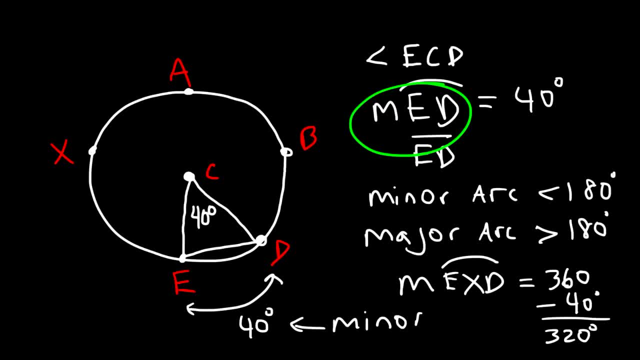 So now, what if we have an arc that has a measure of 180 degrees exactly? So what happens? So notice arc AC. So arc AC has a measure of 180.. And the reason being is because that arc is on the diameter of the circle. 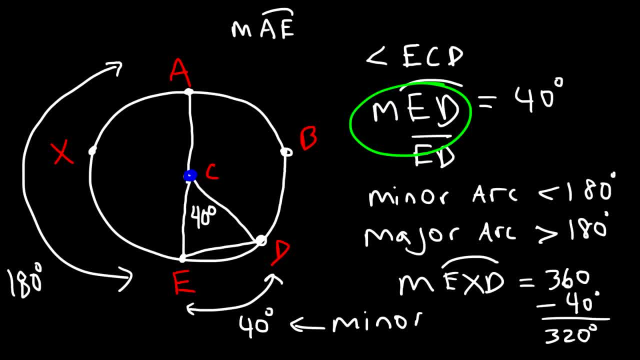 Segment AE. it passes through the center of the circle, which means it's the diameter, And any time you have an arc that is on the diameter of a circle, that arc forms the semicircle, A semicircle, A semicircle. 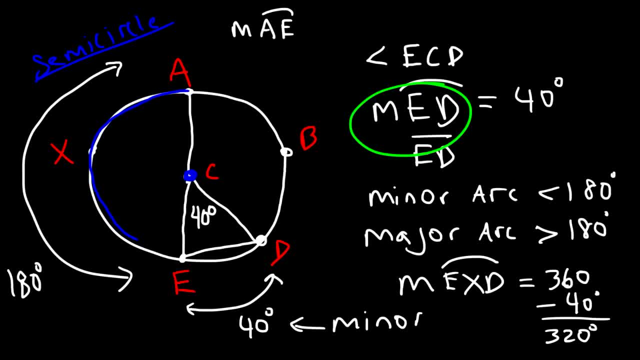 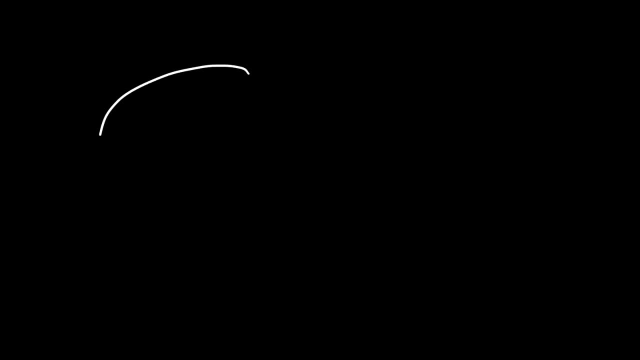 Now let's work on some problems. So let's say, if we have this circle and this is the center and we have a chord between points A and B, This is point C, This is point C, This is point C. 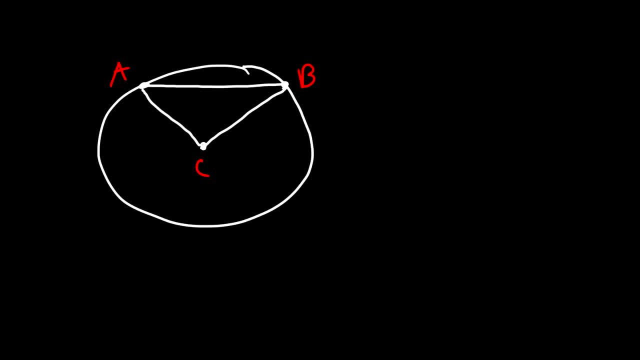 And in this problem, let's say you're given the measure of arc AB. So the measure of arc AB is 100 degrees. With that information, what is the measure of angle A? So feel free to pause the video if you want to try it. 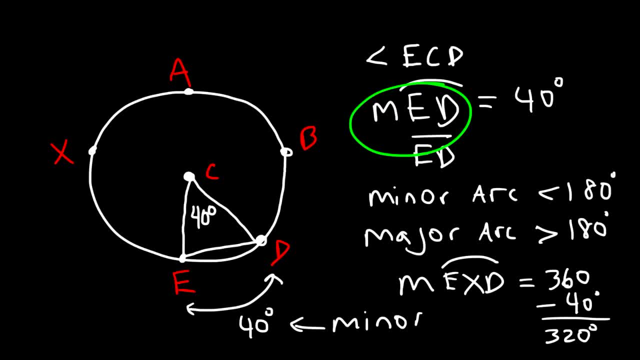 So the measure of arc E, X, D is 320 degrees. So from here all the way to the other side, that's 320 degrees. A full circle is 360.. So we've seen that a minor arc is less than 180, and a major arc is greater than 180. 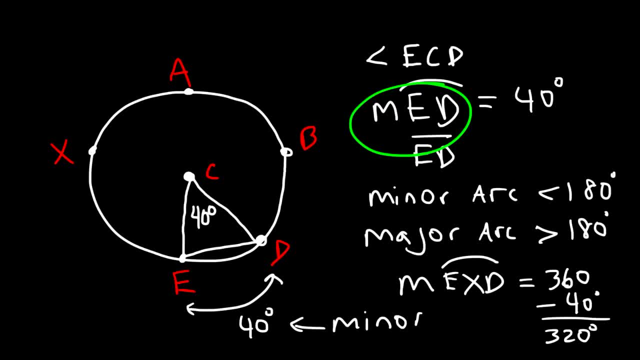 So now, what if we have an arc that has a measure of 180 degrees exactly? So what happens? So notice arc AC. So arc AC has a measure of 180.. And the reason being is because that arc is on the diameter of the circle. 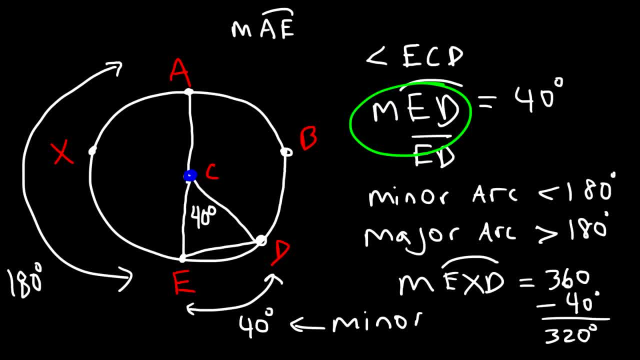 Segment AE. it passes through the center of the circle, which means it's the diameter, And any time you have an arc that is on the diameter of a circle, that arc forms the semicircle, A semicircle, A semicircle. 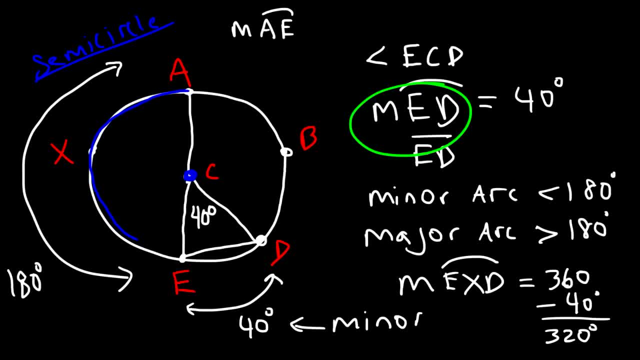 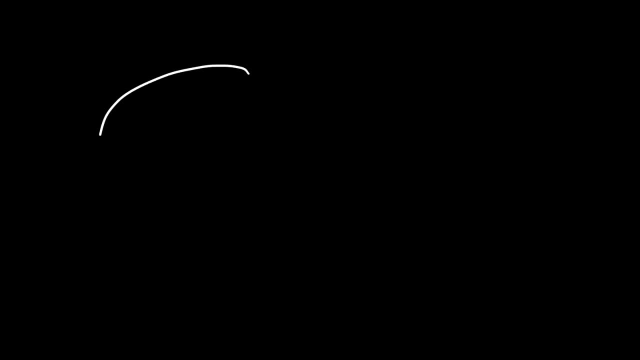 Now let's work on some problems. So let's say, if we have this circle and this is the center, and we have a chord between points A and B, This is point C, This is point C. And in this problem, let's say, you're given the measure of arc AB. 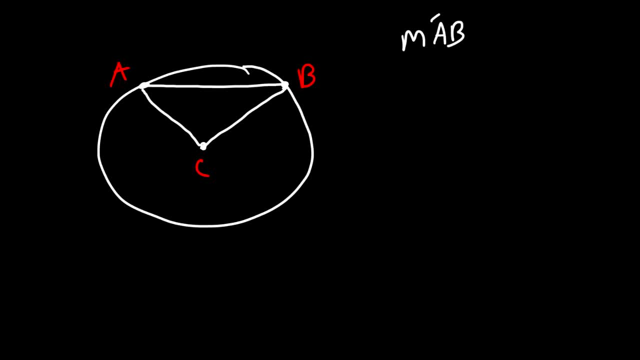 And in this problem, let's say you're given the measure of arc AB. So the measure of arc AB is 100 degrees. With that information, what is the measure of angle A? So feel free to pause the video if you want to try it. 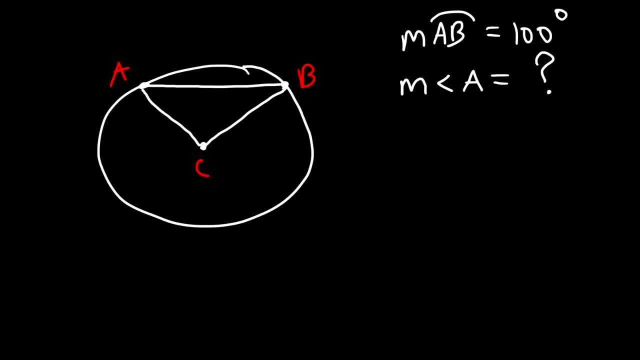 So feel free to pause the video if you want to try it. So arc AB is a hundred degrees. If that's the case, what is the measure of the central angle, The measure of angle ACB, If you recall the intercepted arc and 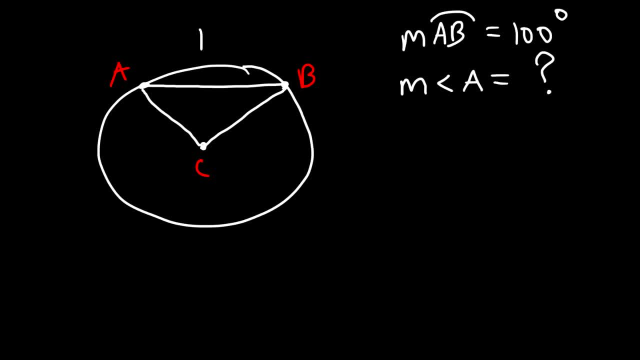 So arc AB is a hundred degrees. If that's the case, what is the measure of the central angle, The measure of angle ACB? If you recall, the intercepted arc and the central angle have the same measure, So angle ACB is also 100 degrees. Now, 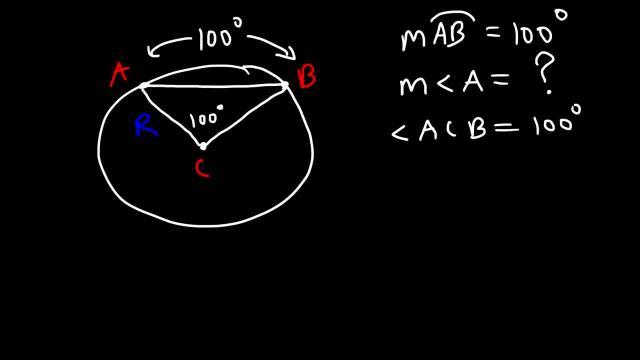 notice that AC is the radius of the circle. The radius of the circle is the distance between the center of the circle and any point on the circle, which means CB is also the radius of the circle. Now, if these two sides are congruent, then the opposite angles must be congruent to each other. We have an 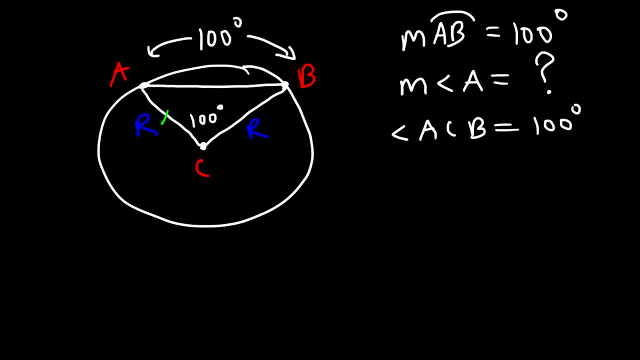 isosceles triangle. So if angle A is X, angle B is X. So now we can calculate the value of X. The three angles of a triangle must add to 180.. So the measure of angle A, B and C must add up to 180.. So A is X, B is X and C is a. 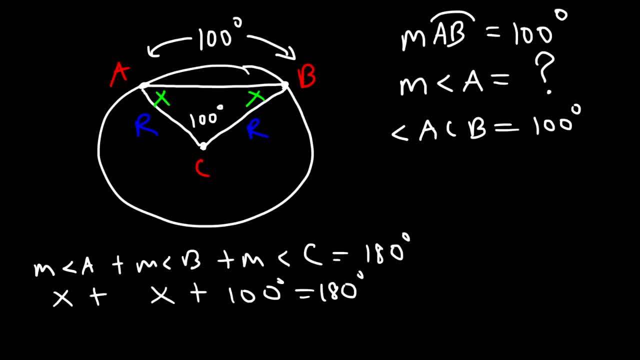 hundred. So 180 minus a hundred is 80, and X plus X is 2X. So 2 X is equal to 80. So if we divide both sides by 20, we have 80.. So 1 minus 1 is 2X. So 1 minus 1 is 2X. So 2X equals 80. So if we divide both sides by 2, 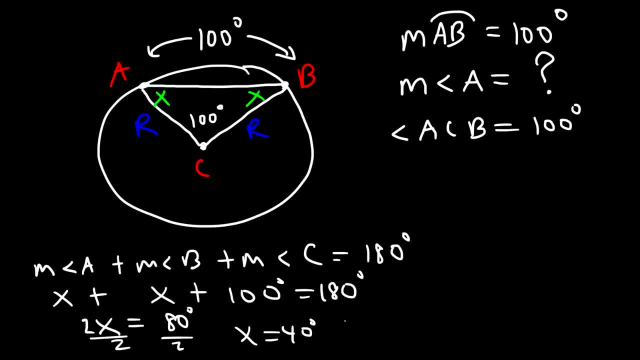 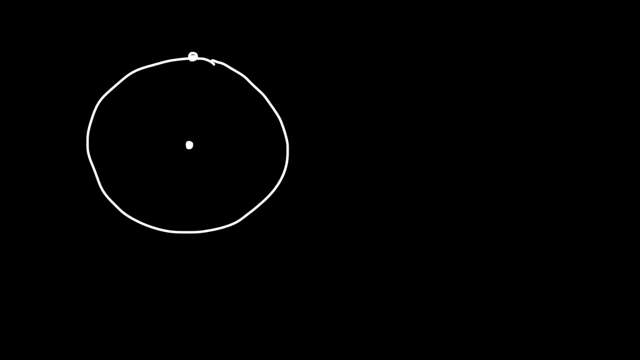 we can see that X is 40. So therefore, the measure of angle A and angle B, they're both equal to 40 degrees. Let's work on another problem. So let's say this is the center and we have two points of interest. So let's call this A, B and center C. Now in this problem, let's say that you're given. 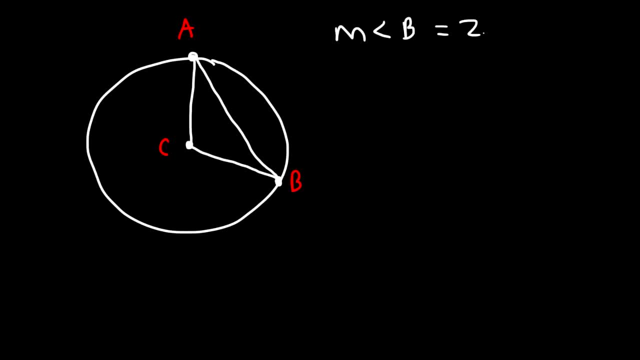 the measure of angle B and it's equal to 20 degrees. And let's say we have another point, point X. What is the measure of angle B? What is the measure of arc AXB? So notice that AXB lies outside of the central angle ACB. So 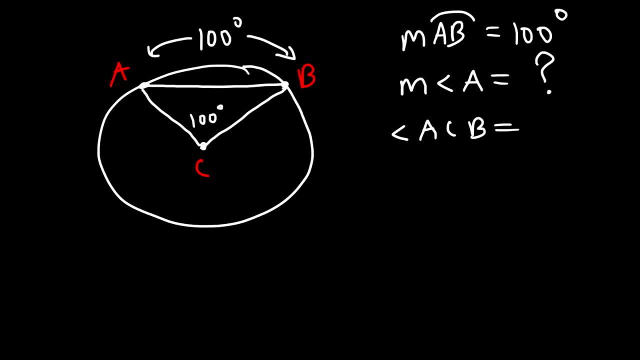 the central angle have the same measure. So angle ACB is also 100 degrees. Now notice that AC is the radius of the circle. The radius of the circle is the distance between the center of the circle and any point on the circle which. 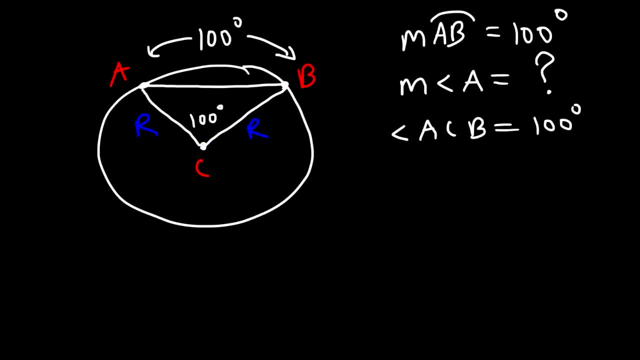 means CB is also the radius of the circle. Now if these two sides are congruent, then the opposite angles must be congruent to each other. We have an isosceles triangle, So if angle A is X, angle B is X. So now we can. 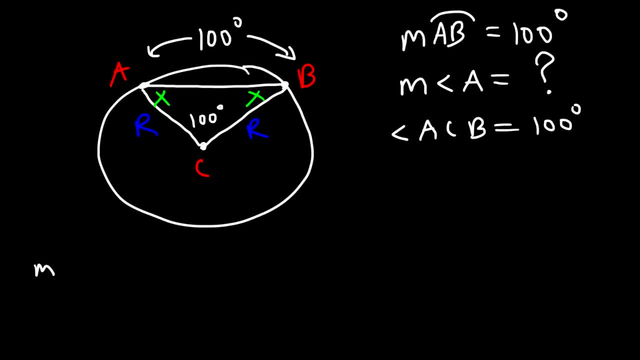 calculate the value of X, The three angles of a triangle must add to 180.. So the measure of angle AB and C must add up to 180.. So A is X, B is X and C is 100. So 180 minus 100 is 80, and X plus X is 2 X. So 2 X is equal to 80.. So if we divide, 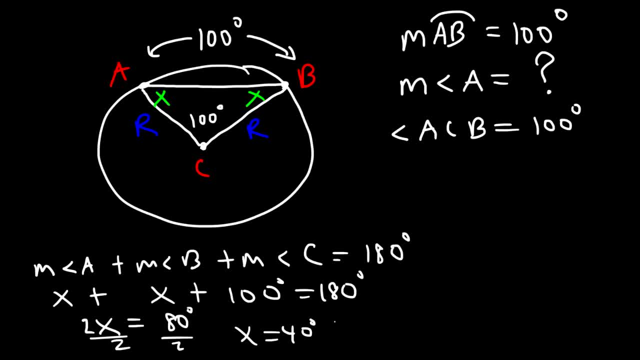 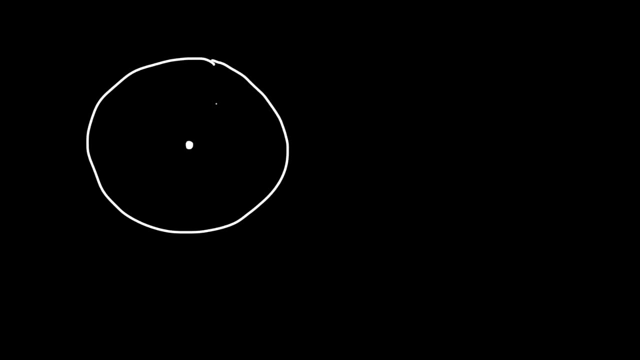 both sides by, we can see that X is 40. So therefore, the measure of angle A and angle B, they're both equal to 40 degrees. Let's work on another problem. So let's say this is the center and we have two points of interest. 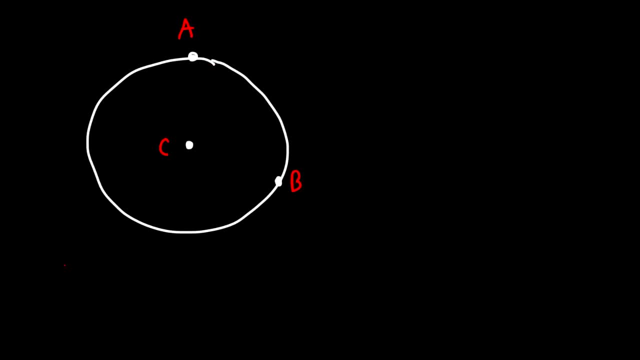 So let's call this A, B and center C. Now, in this problem, let's say that you're given the measure of angle B and it's equal to 20 degrees. And let's say we have another point, point X. 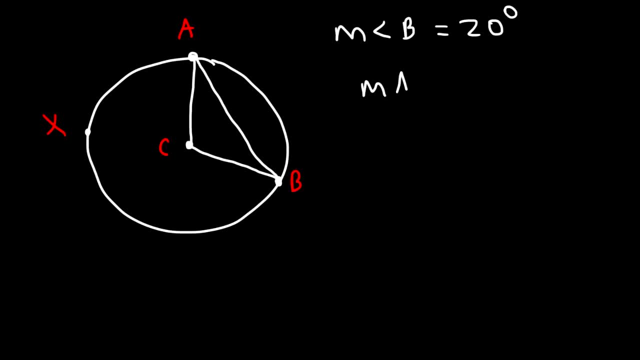 What is the measure of arc AXB? So notice that AXB lies outside of the central angle ACB. So therefore that is a major arc. Calculate the measure of this major arc. Well, since angle B is 20 degrees and CB represents the radius of the circle and AC represents the radius of the circle, 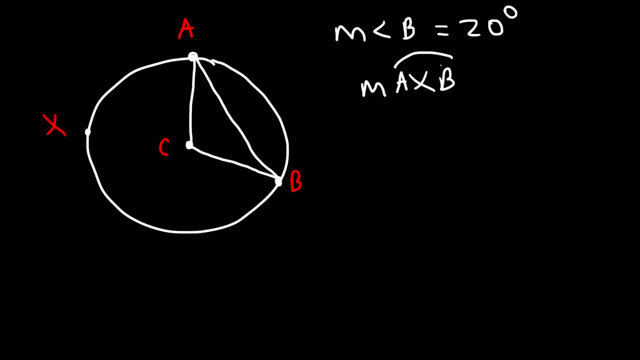 therefore, that is a major arc. Calculate the measure of this major arc? Well, since angle B is 20 degrees and CB represents the radius of the circle and AC represents the radius of the circle, we know that angle B has to be congruent to angle A, So angle A is also 20 degrees. So now we can calculate the measure of angle C. Let's call it X. So X plus 20 plus 20 has to add up to 180.. 20 plus 20 is 40. And 180 minus 40 is 140.. So that's the measure of angle ACB. 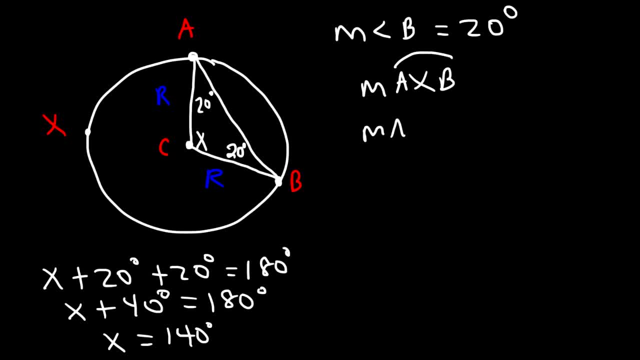 Which means that arc AB has to be 140 as well. If this is 140, the central angle, then the intercepted arc must also be the same. So now that we have the measure of arc AB, we can calculate the measure of arc AXB, And so it's going to be 360 minus 140. 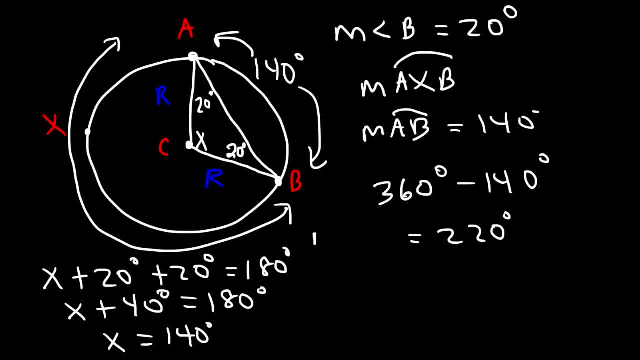 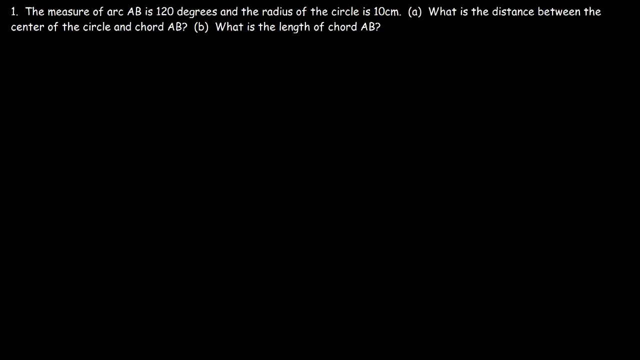 And so that's going to be 220 degrees. So that's the measure of arc AXB, the major arc, And so that's it for this problem. Try this problem. The measure of arc AB is 120 degrees and the radius of the circle is 10 centimeters. What is the distance between the center of the circle and chord AB? 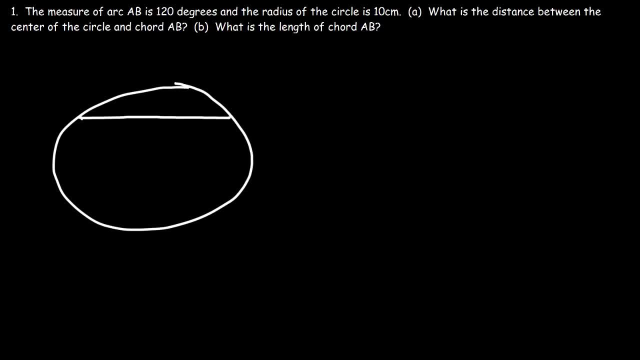 So let's draw a circle And let's say: this is 120 degrees the cord, and here's the center of the circle. So this is AB and this is point C. Now let's turn this into a triangle. So the measure of arc AB is 120 degrees. So that means that 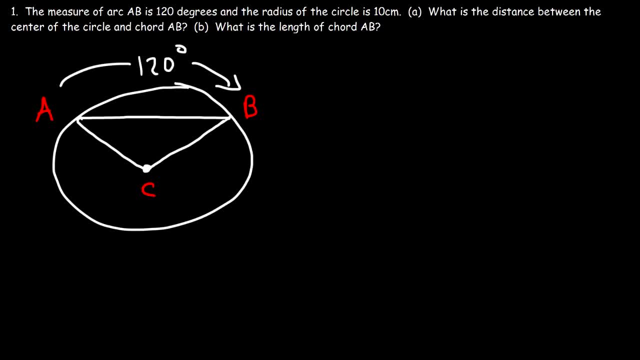 the central angle, angle ACB is also 120.. So if we want to, we can now calculate angle A and B. So if this is X and that's X, we can say that 120 plus X plus X, that's equal. 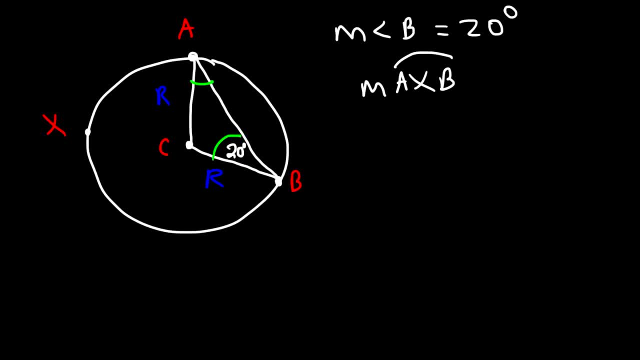 we know that angle B has to be congruent to angle A, So angle A is also 20 degrees. So now we can calculate the measure of angle C. Let's call it X. So X plus 20 plus 20 has to add up to 180.. 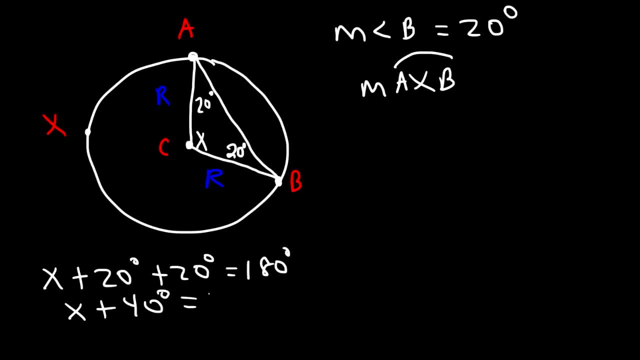 20 plus 20 is 40. And 180 minus 40 is 140. So that's the measure of angle ACB, which means that arc AB has to be 140 as well. If this is 140, the central angle. 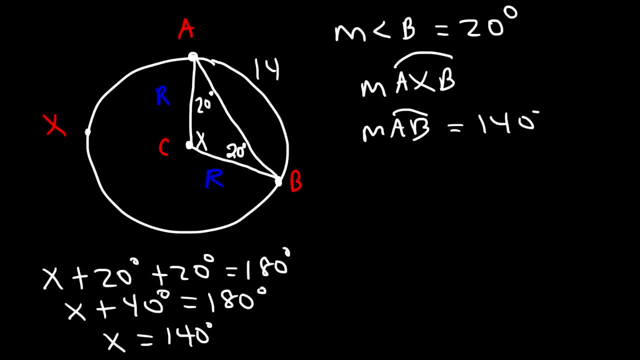 then the angle A is also 140.. So that's the measure of angle ACB, which means that arc AB has to be 140 as well, And the intercepted arc must also be the same. So now that we have the measure of arc AB, 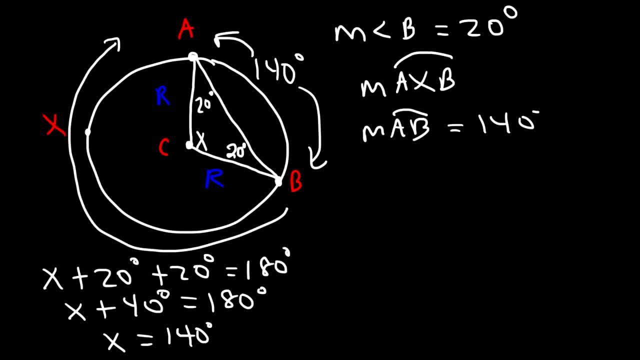 we can calculate the measure of arc AXB, And so it's going to be 360 minus 140., And so that's going to be 220 degrees. So that's the measure of arc AXB, the major arc, And so that's it for this problem. 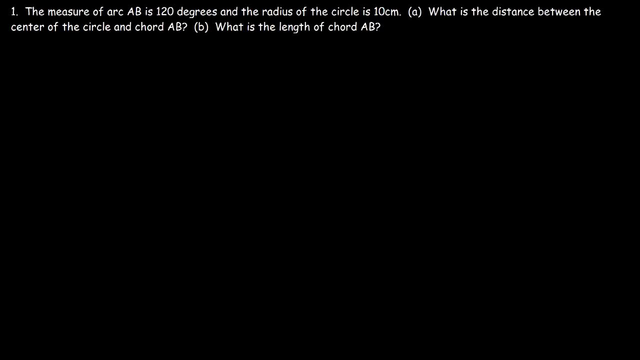 Try this problem. The measure of arc AB is 120 degrees And the radius of the circle is 10 centimeters. What is the distance between the center of the circle and chord AB? So let's draw a circle And let's say this is the chord. 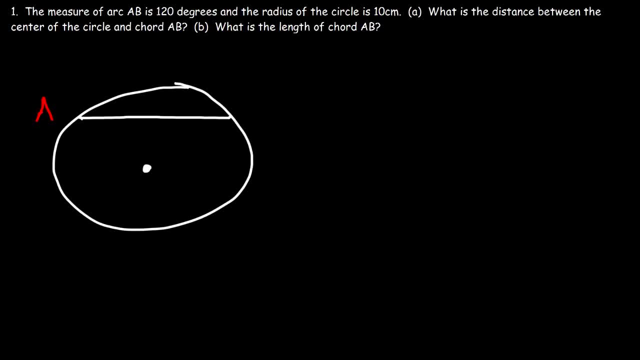 And here's the center of the circle. So this is AB and this is point C. Now let's turn this into a triangle. So the measure of arc AB is 120 degrees. So that means that the central angle, angle ACB, is also 120. 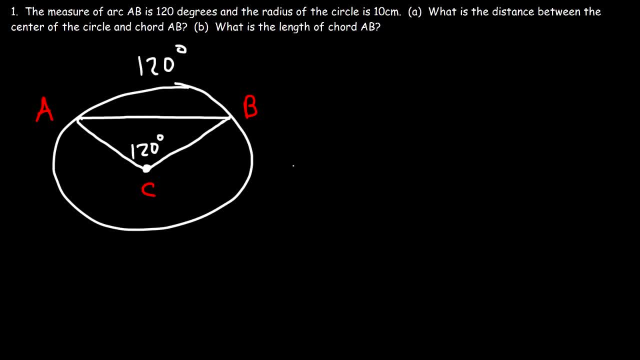 So, if we want to, we can now calculate angle A and B. So this is X and that's X. We can say that 120 plus X plus X, That's equal to 180.. So 180 minus 120, that's 60.. 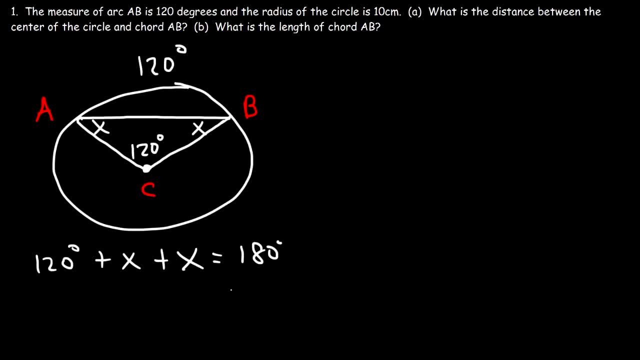 to 180.. So 180 minus 120, that's 60. And X plus X is 2X. So 60 divided by 2 is 30. So angle A and angle B, they're both equal to 30 degrees. So now, what should we do at? 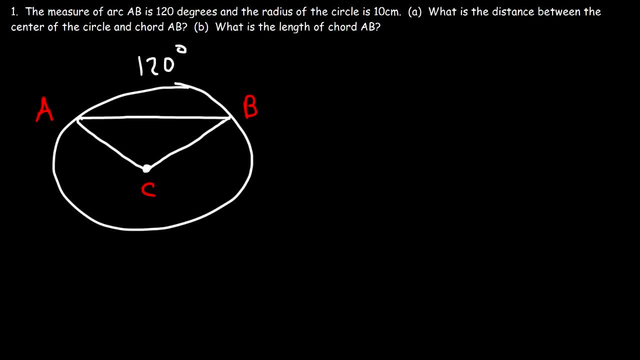 this point. So this is 30,, this is 30, and if I draw a line between- let's call this D. So if I could draw a line between the cord and the center of the circle and do so in such a way that this is the right angle, then we can see that this has to be 60 and this 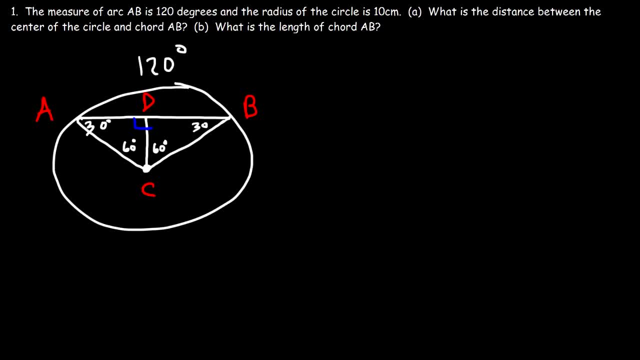 is 60, so that they add up to 120.. Now we're told that the radius of the circle is 10 centimeters. So AC is 10 and BC is 10.. Now in part A we need to calculate the distance between the: 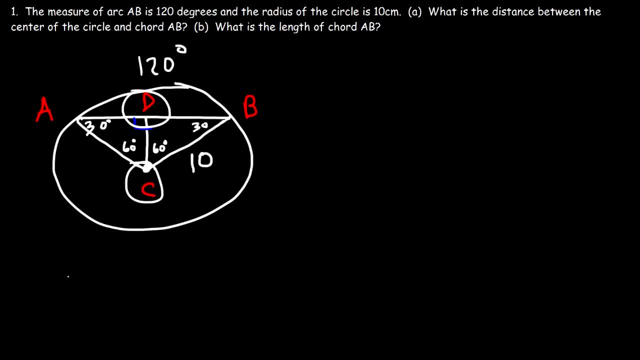 center of the circle and cord AB. So we got to find the length of segment CD. How can we do so, given the radius? So notice that we have a 30-60-90 triangle And we have the hypotenuse, which is 10.. Now for a 30-60-90 triangle. if the hypotenuse is 2, then the 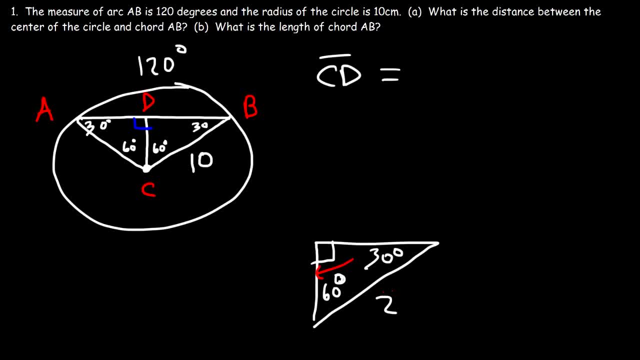 side across the 30, that's going to be 20.. So we're going to have to calculate the length of segment CD. That's going to be half of 2. It's 1., And the side across the 60, it's. 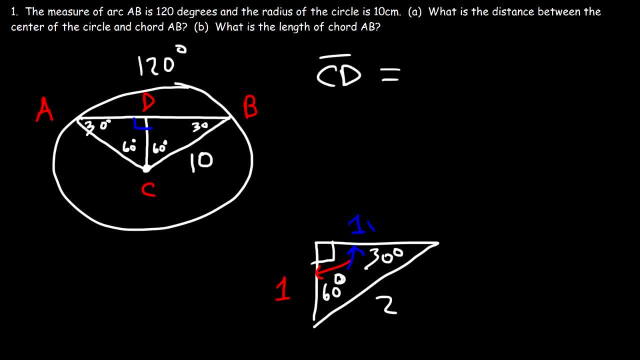 going to be. whatever this number is, times the square root of 3.. So therefore, if this is 10, then the side across the 30 has to be half of 10, which means it's 5 units long. So therefore, CD is equal to 5.. So that's the answer to part A. It's 5 centimeters Now. 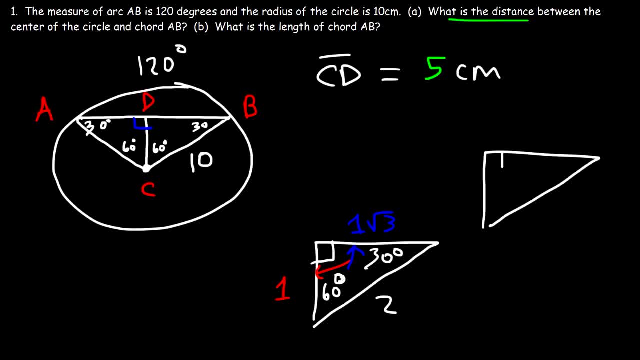 if CD? I'm going to draw because this is small- If CD is 5, what's DB? So across the 60 degree angle that side is going to be, whatever this number is, times the square root of 3.. So it's. 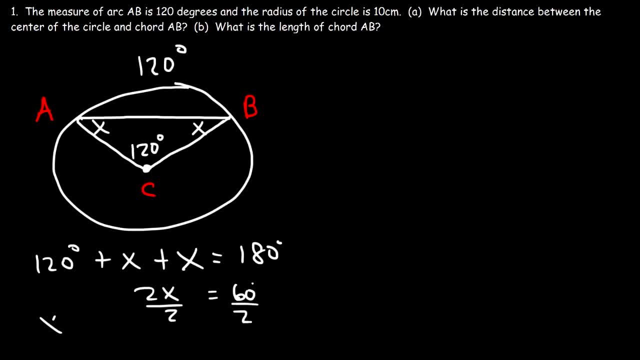 And X plus X is 2X. So 60 divided by 2 is 30. So angle A and angle B: they're both equal to 30 degrees. So now, what should we do? at this point, We're going to draw a line between the center of the circle and the chord AB. 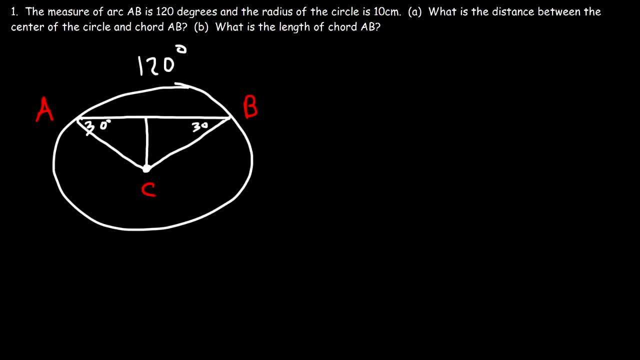 So this is 30.. This is 30. And if I draw a line between- let's call this D, So if I draw a line between the chord and the center of the circle and do so in such a way that this is the right angle, then we can see that this has to be 60 and this is. 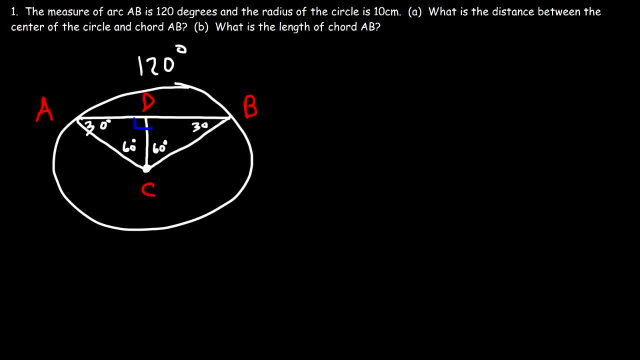 60. So that they add up to 120.. Now we're talking about the angle AB. Now we're told that the radius of the circle is 10 centimeters. So AC is 10 and BC is 10.. Now in part A we need to calculate the distance between the center of the circle and chord. 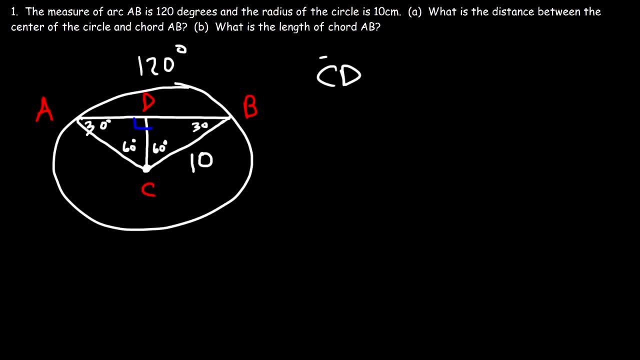 AB. So we got to find the length of segment CD. How can we do so, given the radius? So notice that we have a 30,, 60,, 90 triangle And we have the hypotenuse, Which is 10.. 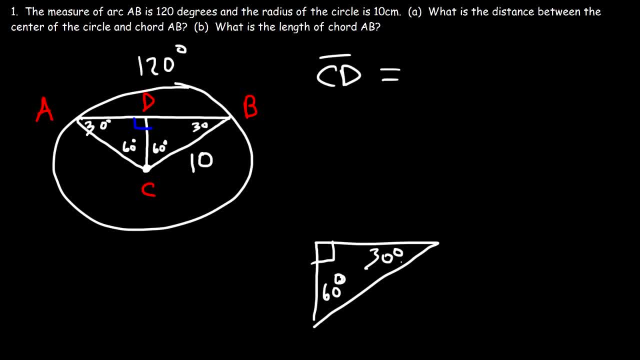 Now for a 30, 60, 90 triangle. if the hypotenuse is 2,, then the side across the 30,, that's going to be half of 2.. It's 1., And the side across the 60, it's going to be whatever. this number is times the square. 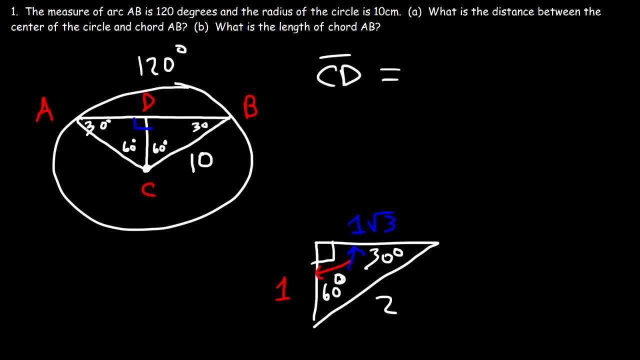 root of 3.. So therefore, if this is 10, then the side across the 30 has to be half of 10.. Which means It's 5 units long. So therefore, CD is equal to 5.. So that's the answer to part A. It's 5 centimeters. 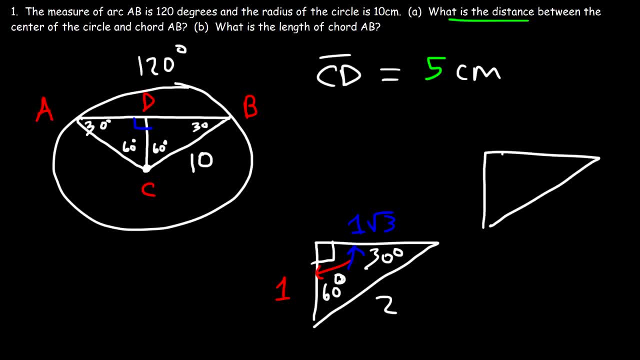 Now, if CD- let me redraw because this is small- If CD is 5, what's DB? So across the 60 degree angle that side is going to be whatever this number is, times the square root of 3.. So it's 5 square root of 3..